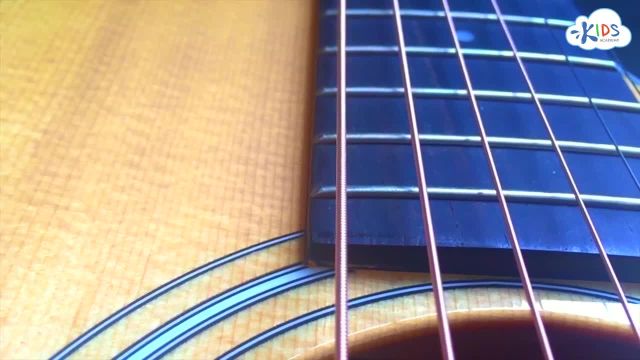 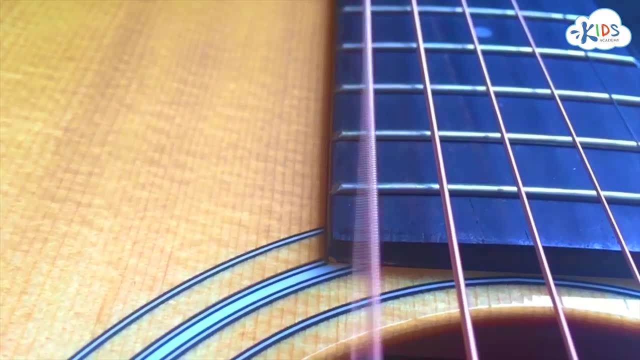 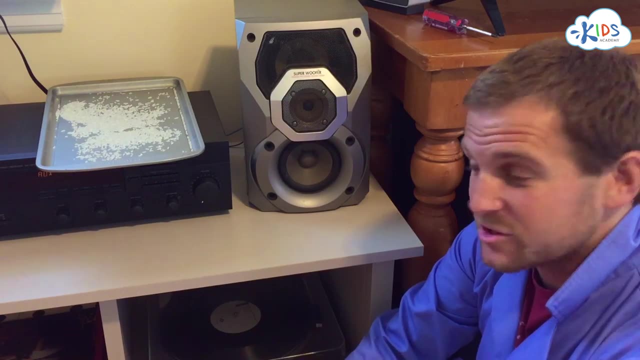 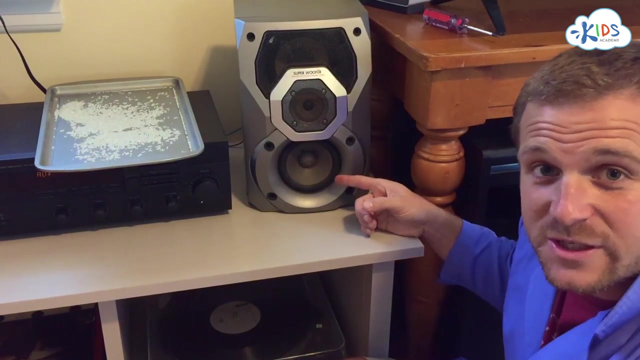 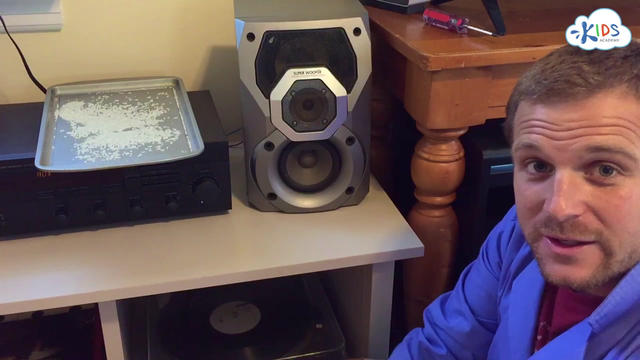 Musical instruments like guitars take advantage of these vibrations. Watch as this guitar string vibrates rapidly to make noise. We mentioned that sound is vibrations, and sound coming out of a speaker or your headphones is no different. You can see on this speaker. we have a cone here. Now what this cone is going to do when electricity is run through it is it'll bump back and forth and cause vibrations to come out and make sound for us. 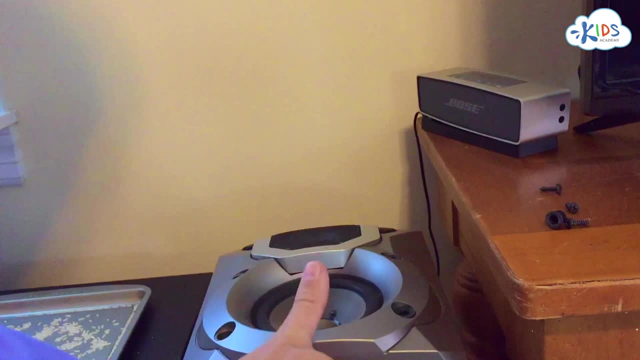 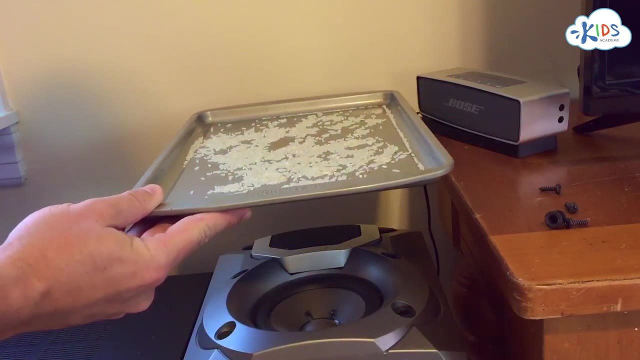 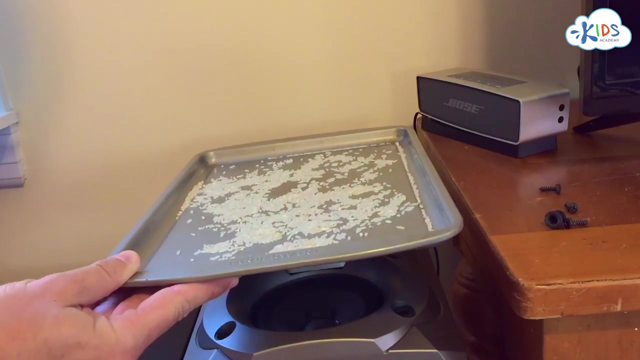 You can see here that I've laid the speaker on its back so that the cones are pointing up. Now I'm going to hold this tray of rice Just above the speaker. I'm not going to touch the speaker because I want to show that the vibrations are going to travel through the air and vibrate our rice. 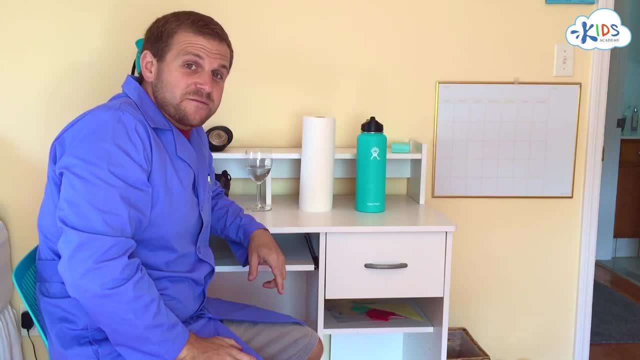 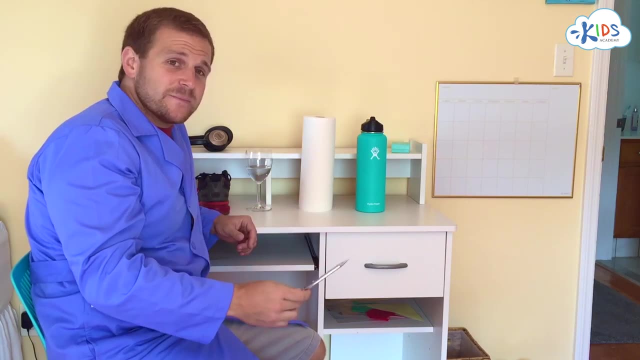 For the most part, the harder an object is, the better it's going to vibrate. So we have a couple of objects here And I'm going to be using this metal pencil to bang against them and let's see what kind of sounds we can get out of them. 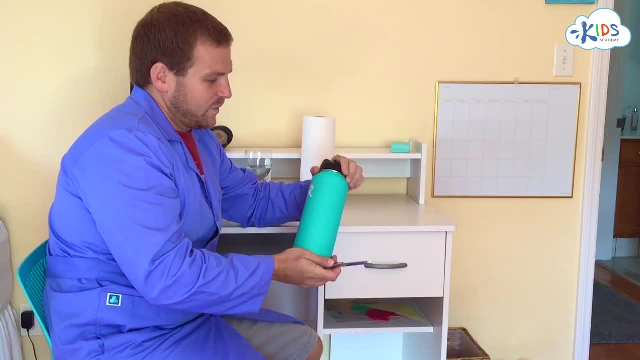 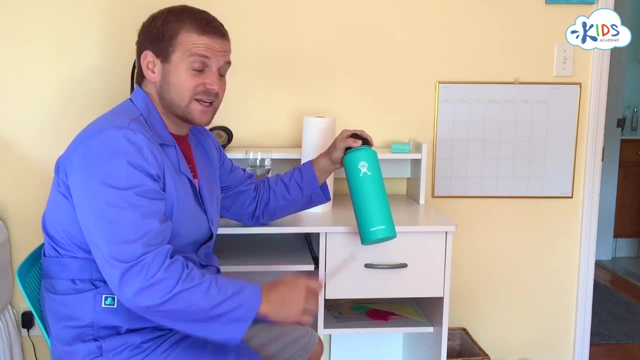 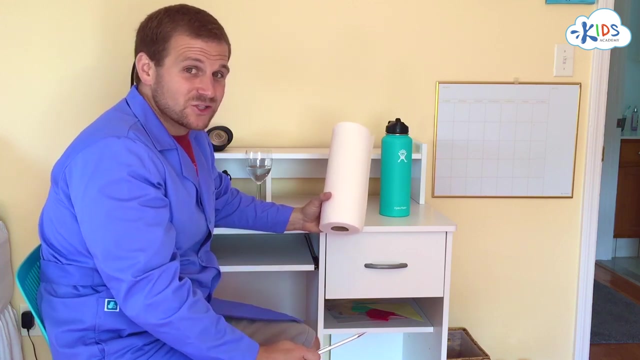 The first one is a metal water bottle. Now, metal is a very hard substance, so we should get a pretty good sound, A lot of vibrations. I can actually feel the vibrations in my hand Now. paper towels are very soft, so we really shouldn't get a good sound, a big sound, from this one. 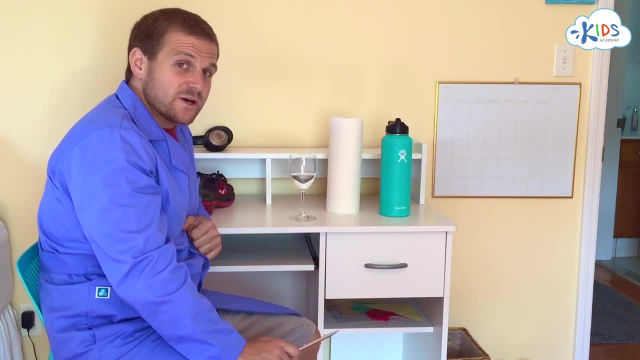 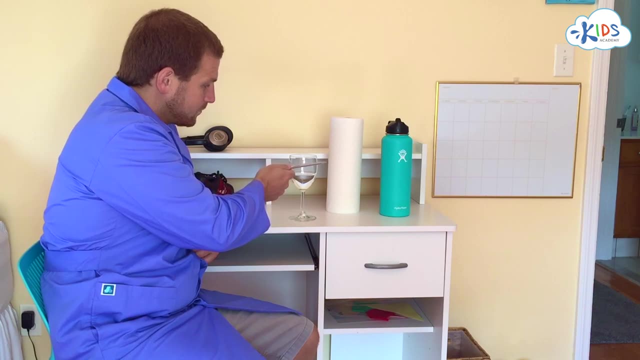 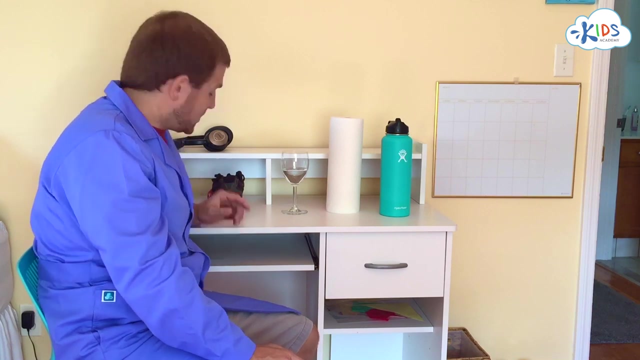 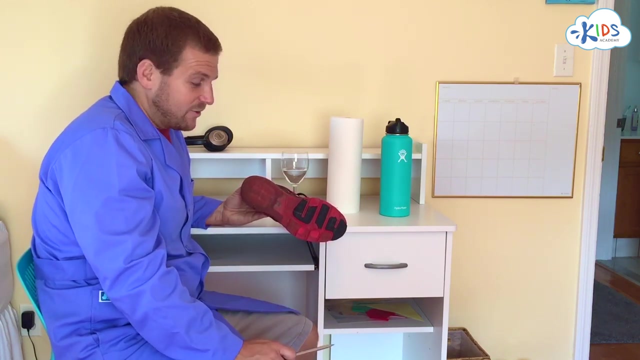 Not much. The glass is really hard, so we should get a good sound from this. Now I'm going to be careful as I do this. We do get a pretty good sound. Some things are actually made to absorb vibrations. The rubber on the bottom of your shoe is made to absorb the vibrations from you stepping on the ground all day long to make it softer on your feet. 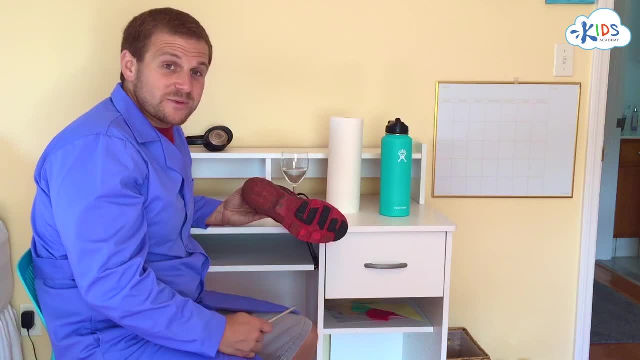 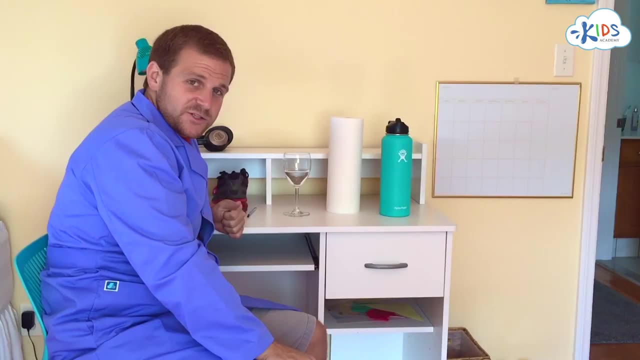 So it should, just like it absorbs those vibrations from the ground, absorb the sound from the pen, Not a whole lot of sound. Here's a neat trick you can do with your parents' permission. Get a glass like this and put some water in it. 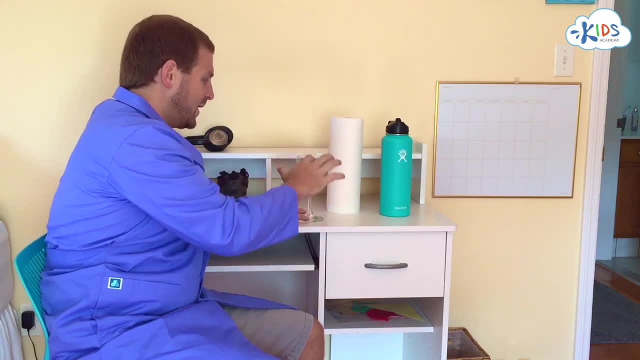 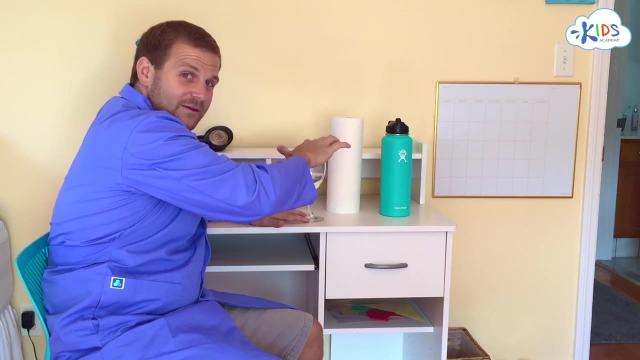 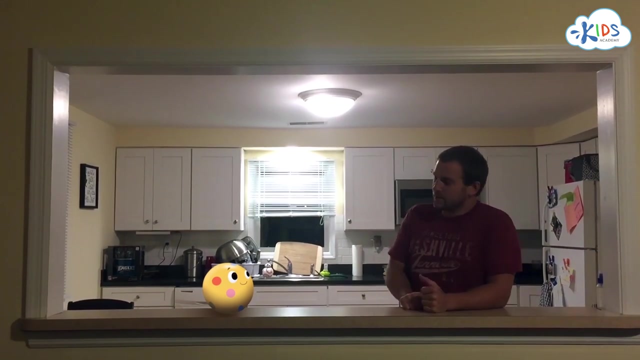 Get your finger wet and then rub it around the outside of the glass. As you rub it, you should cause the glass to vibrate and you'll hear a big noise. So, Molly, We've talked a lot about sound. Sound is energy.